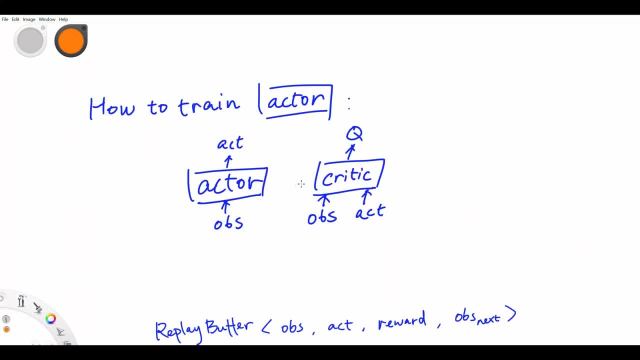 and the next observation. Now let's see how to train the actor network. That's pretty easy. Assume that we already have a well-trained Q Network And what we are going to do is to move the actor network just under the Q Network and then fit into the real-world observations, We can have a. 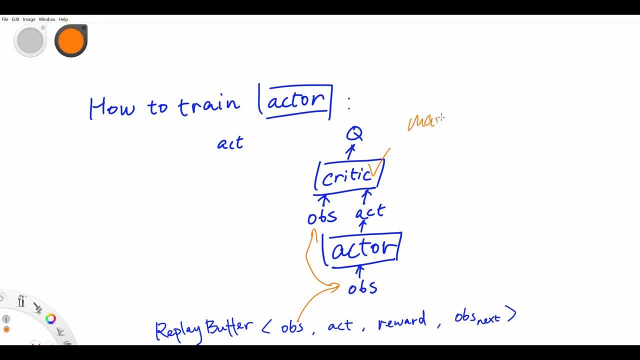 Q value. What we are going to do next is to maximize the Q value output, or to say, minimize the minus Q. In this way, we can have the extra network trained as well. Next is how to train the credit. We already know that Q equals the reward plus a discounted. 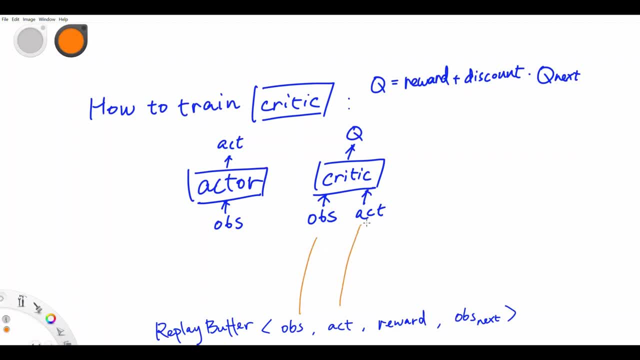 Q next. What we can see is that we already have the Q value here. We also have the reward. What we want is the Q next. So what we are going to do is to reuse this credit network. I will just make a copy and move it here, And we are also going to use this. 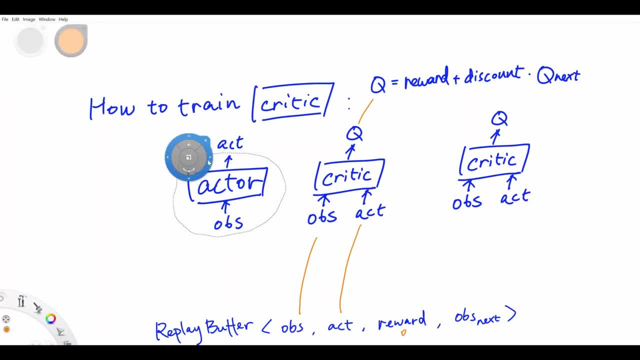 actor network. Let's move it just under the credit network. So what we are going to do is to fit in the next observation and just mark it next. next, And the output from this actor is the optimal action for the next observation, Let's mark: 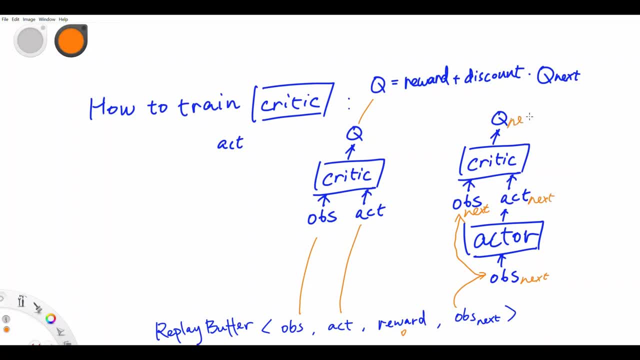 it too. So what we get now is the next Q, As we can see here, is that we already have the Q. next the reward and the Q- How we are going to train. the credit is that we are going to make the both sides of the equation getting. 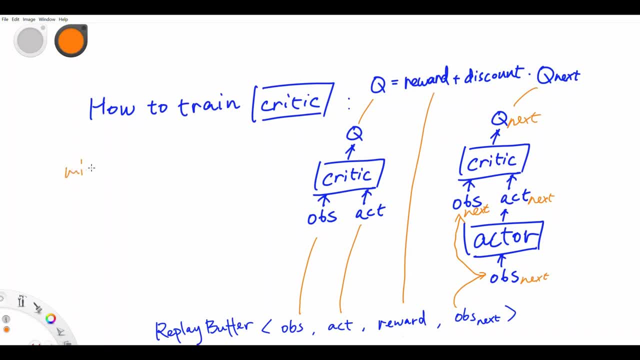 closer, which means to minimize the difference between Q and reward plus discounted Q. So what we are going to do next is to minimize the difference between Q and reward plus discounted Q. Next Q. A problem here is that if these two credits comes from the same network, then the update. 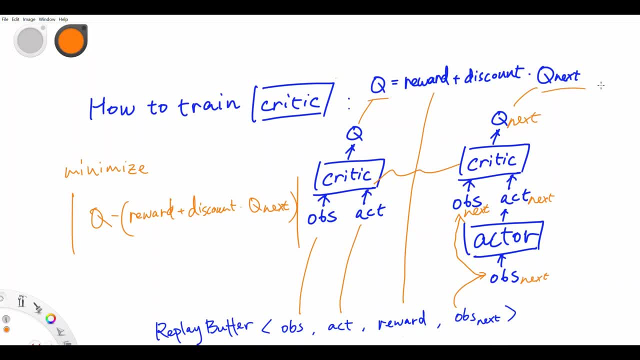 of this network will make the Q and Q next change in the same time, which makes the training process more unlikely to converge, such that DDPG is also using a target network. to solve this problem, To implement the target network, we are going to use the target network. 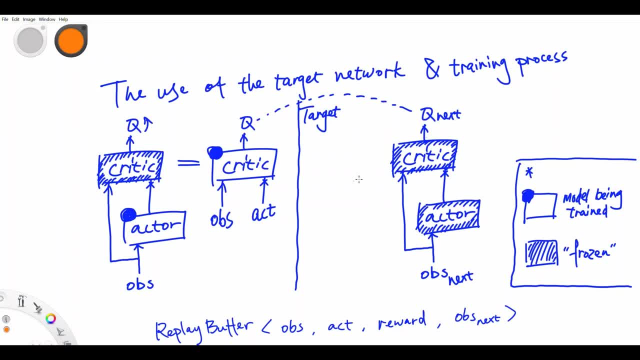 The DDPG has two sets of actor and credits. When training the actor, it freezes the credit and feeds in the observation, making the Q getting larger. So the actor is getting updated. When training the credits, it feeds in the observation and action also feeds the next. 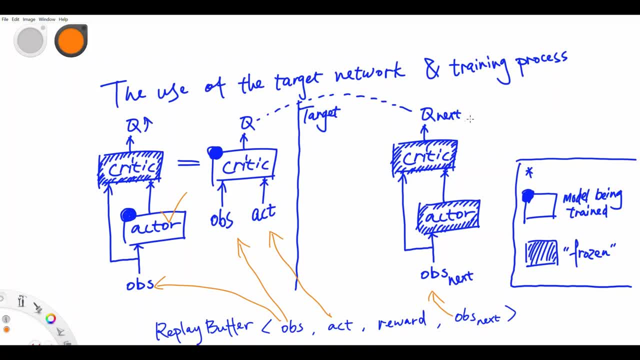 observation to the target network: getting the Q next And trying to make the Q in the target network. get the Q next, Make the Q equals to the reward plus the discounted Q next, And so the credit network is also getting updated. And finally, the trained module parameters will be slowly updated to the target network. 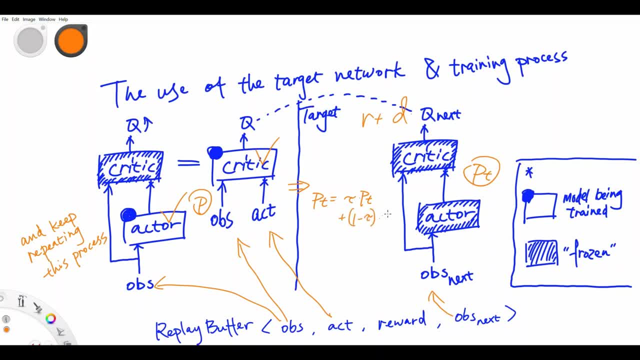 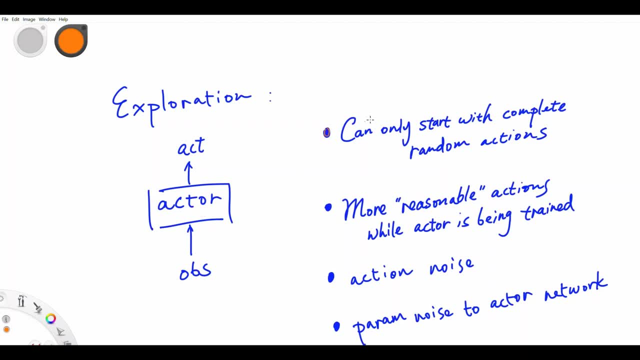 using a moving average style. Finally, the exploration. It's obvious that the model is only capable of making totally random actions in the beginning. So if you are using RL to play a game, generally the player will just kill itself instantly when the game starts. 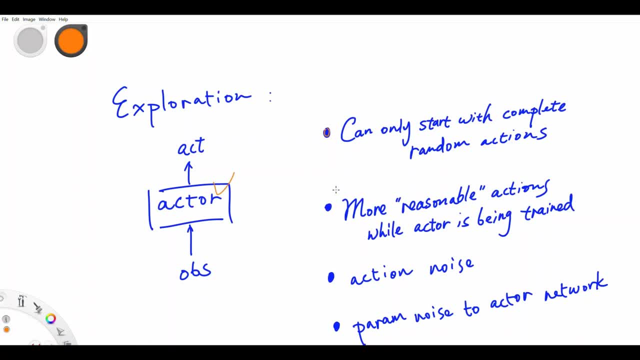 While the actor is being trained, the player is more likely to make reasonable actions, which will unfold more situations. Moreover, action noise can be added to the output of the actor, and parameter noise can also be directly injected into the action, Just like the evolution strategy. 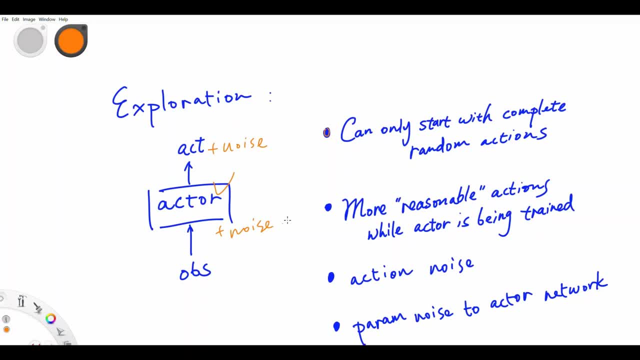 Hello, thanks for watching. This is my fourth video with a lot of technical issues. The background, noise and volume is keep changing. Plus, my English is not that good, So I have to record again and again. But however it is, hopefully it can be useful and see you soon in the next video. 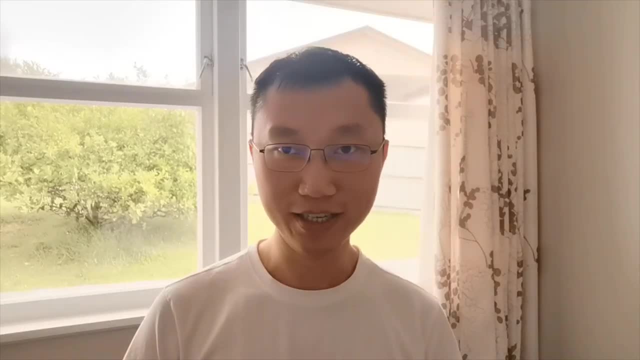 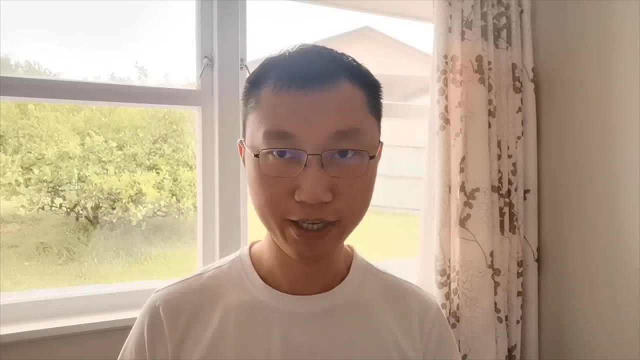 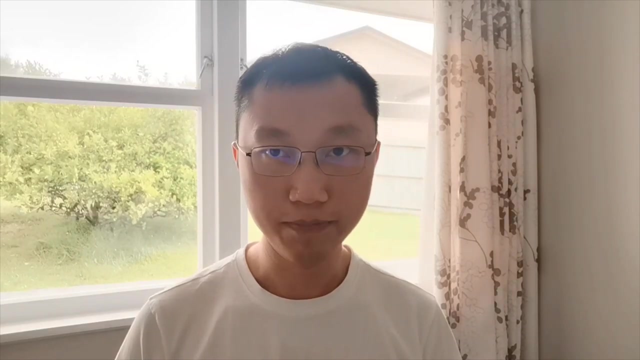